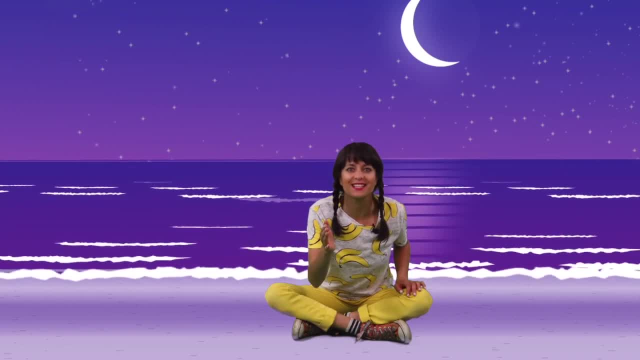 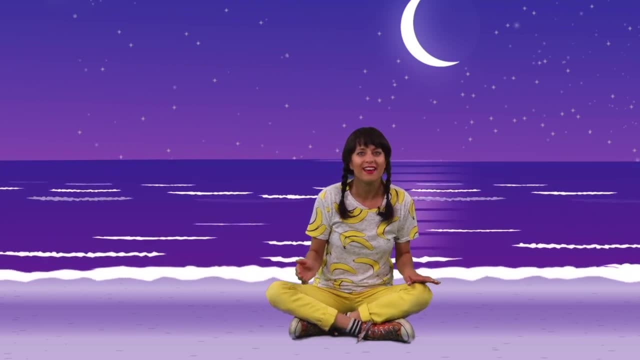 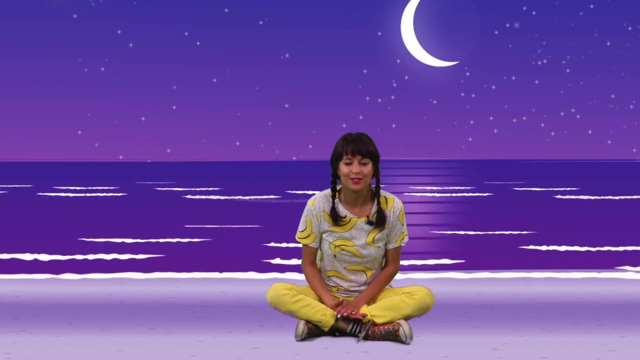 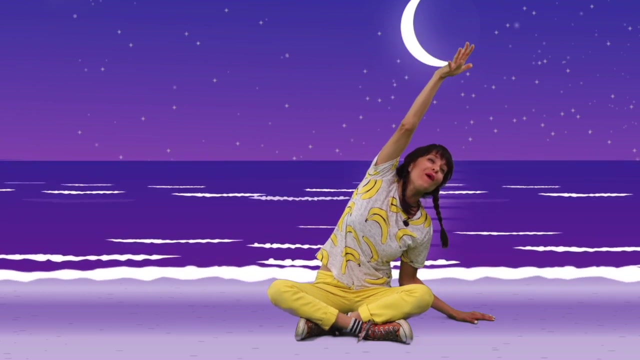 And listen. Do you hear the crickets and the waves crashing? There's so many things to hear and look around and see. Well, first, before I go to bed, I like to do a few things like yoga and breathing and gratefulness. So let's start with some yoga. Let's put our hand on the side and turn our body into a crescent moon, Stretch your arm out all the way, Take a deep breath in through your nose and exhale, and come all the way back. 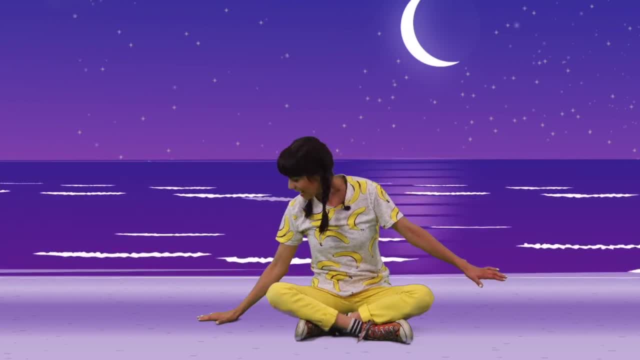 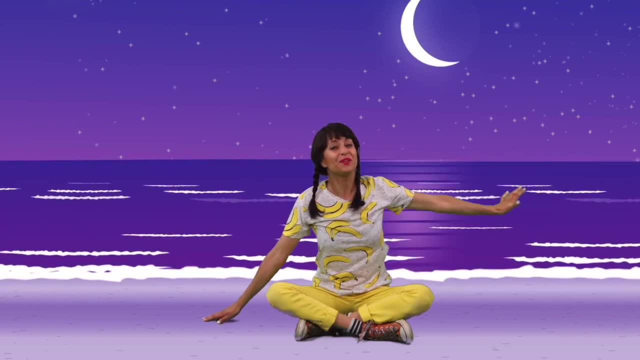 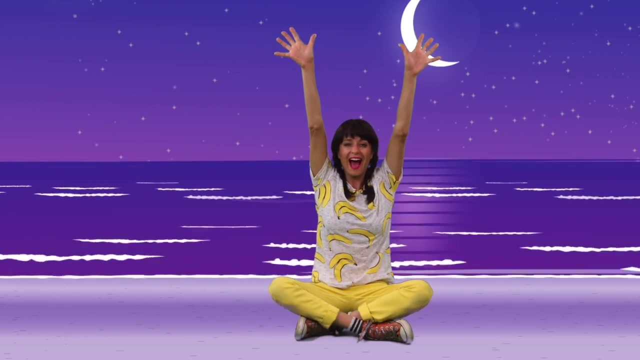 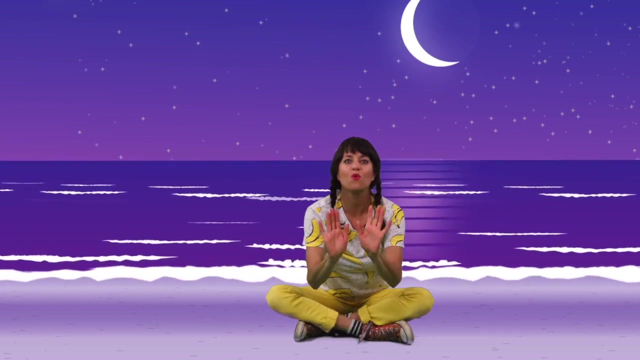 Let's try it again on the other side. Put your hand in the sand, Take a deep breath in and exhale it out. Those are good crescent moons. Hey, you know we could also do a stretch like the waves. So stretch your arms up really high, Take another deep breath in and crash your ways down to the sand. Let's try it again. Take another deep breath in, Stretch your arms up and out. 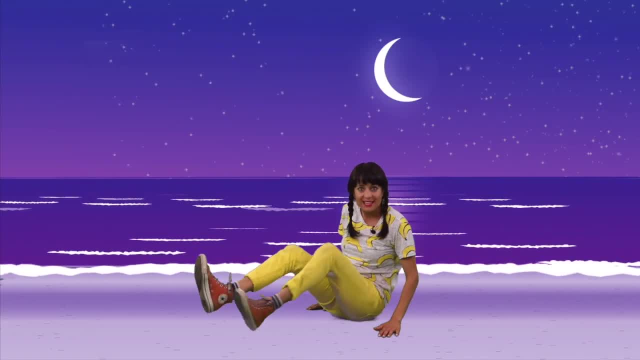 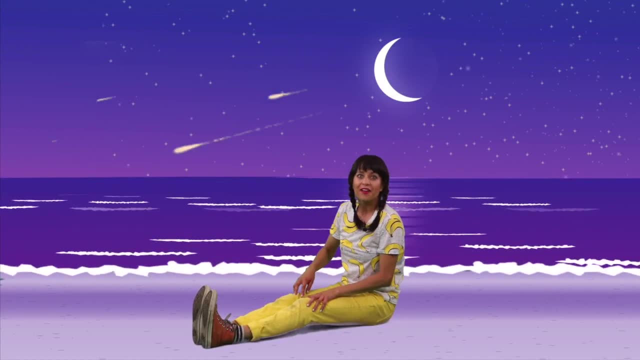 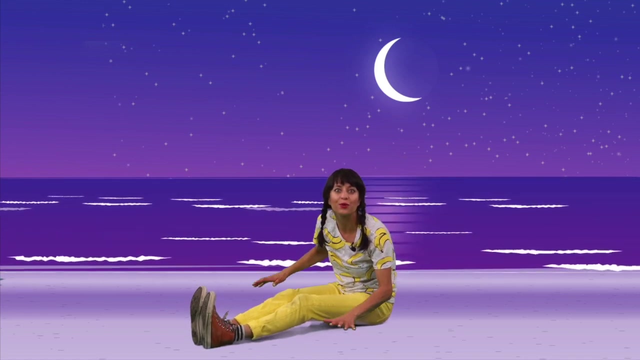 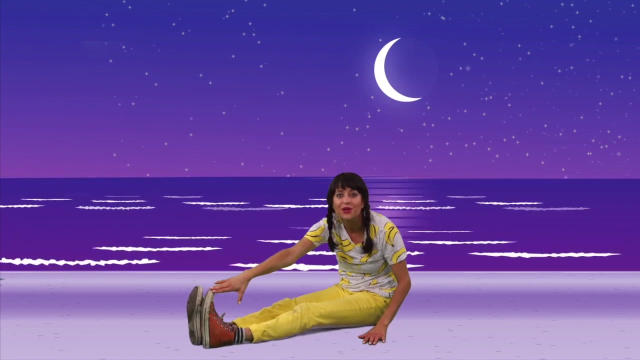 Now let's see if we can stretch our legs out. Can you do that? Stretch them all the way out. You can even get your wiggles out too. Oh, look a shooting star. Wow, No way Did you see it. Maybe we could reach behind us and try to grab one from the sky. So stretch your body and reach, Pull it out of the sky and see if you can bring it all the way across onto your toe. And let's stretch this side, Reach and grab a shooting star and bring it all the way up. 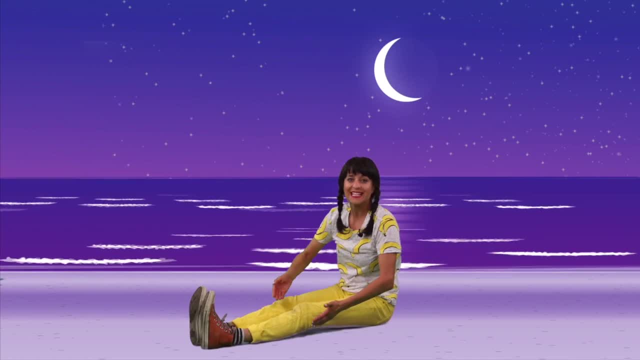 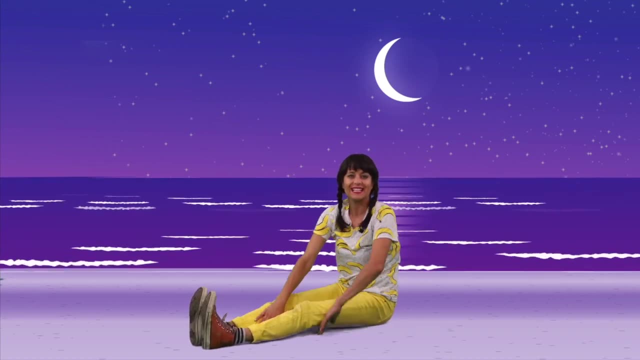 All the way across and put it on your toe. Let's try it again. Take a deep breath in and exhale it all the way back down to your toes. Let's try it again: Deep breath in and all the way across our body. 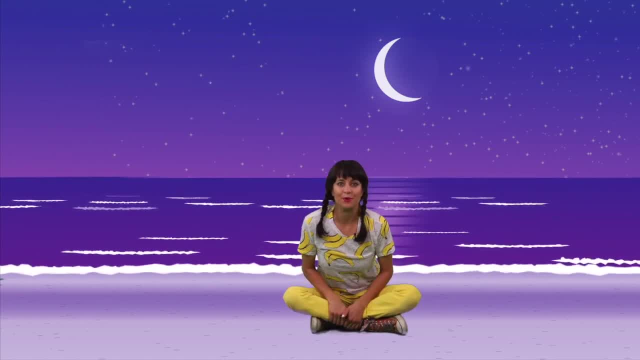 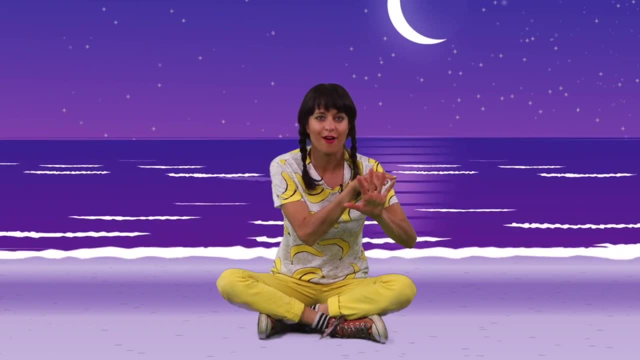 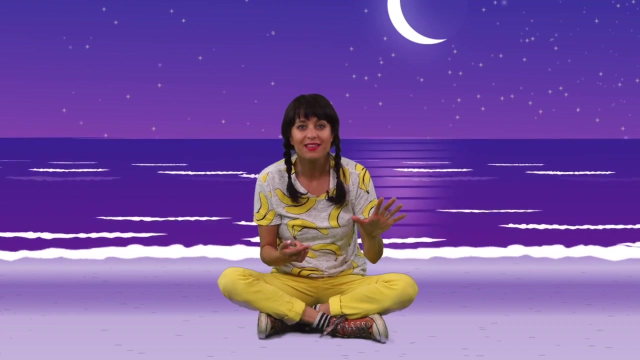 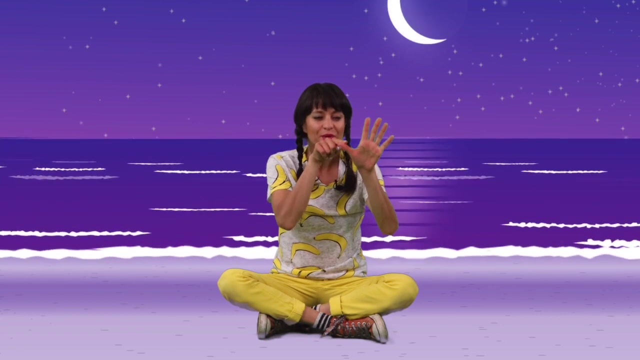 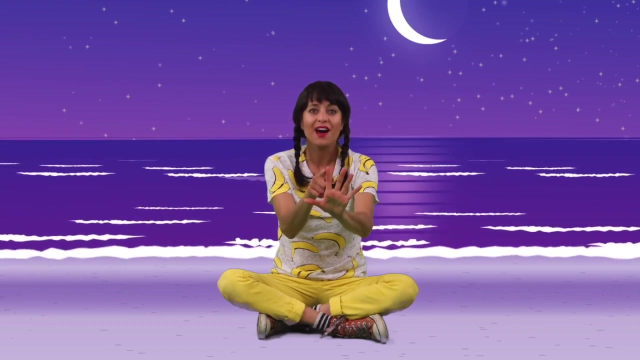 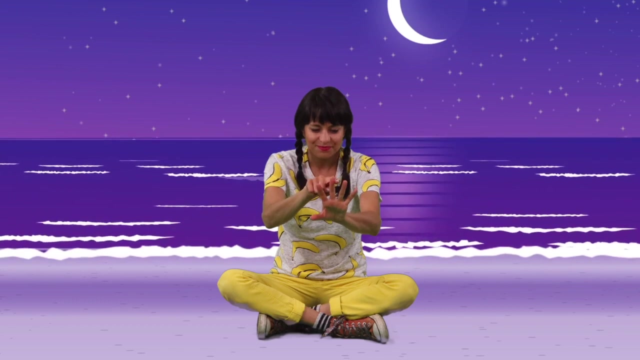 Well, now that we did our yoga poses, let's see if we can do our breathing. So, can you take your hand out, just like this, and let's count how many fingers we have? One, two, three, four, five, And we're going to bring our fingers into waves that we can surf up and down, And we're going to use our breathing to help us go up the wave. Now take a deep breath in through your nose and exhale out and go down the wave. That's it. Try it again. Take a deep breath in and exhale to go down. Try it again: Deep breath in and out. That's it. You're doing great. 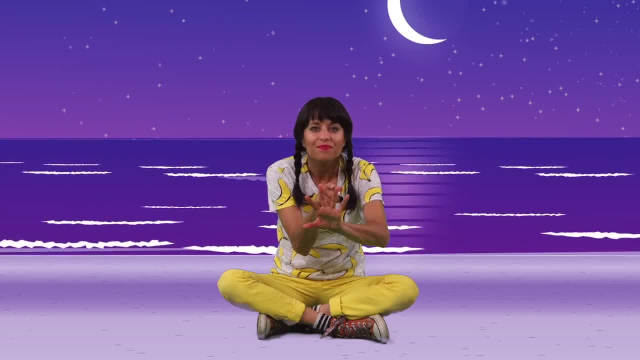 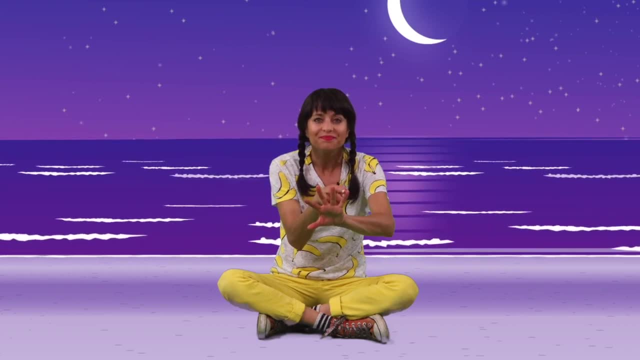 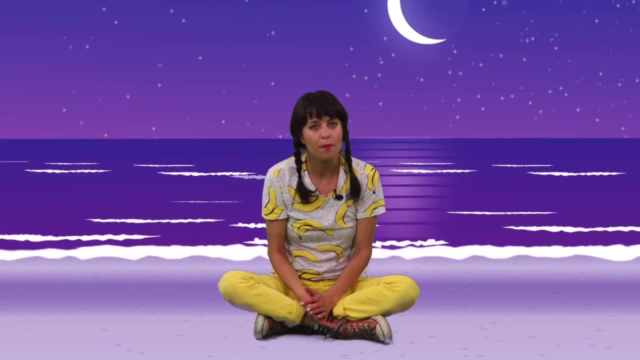 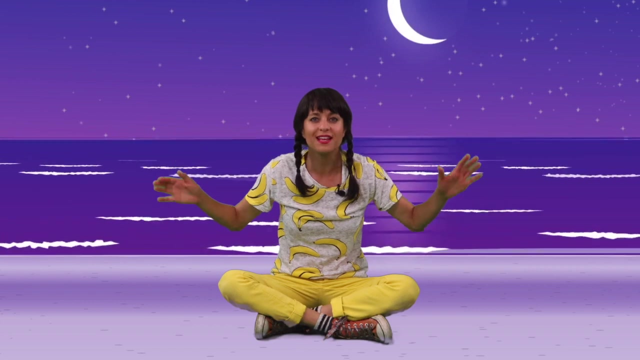 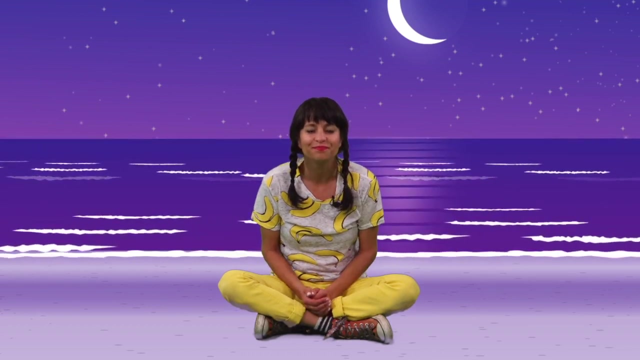 Deep breath in through your nose To go up and breathe out, to go down. One more time: Deep breath in and breathe out. That's it Now. at nighttime, it's so important to breathe in through our nose and out through our nose too. It helps to get all the air around us really deep into our body, which is so important. So let's try it again: Take a deep breath in and exhale. 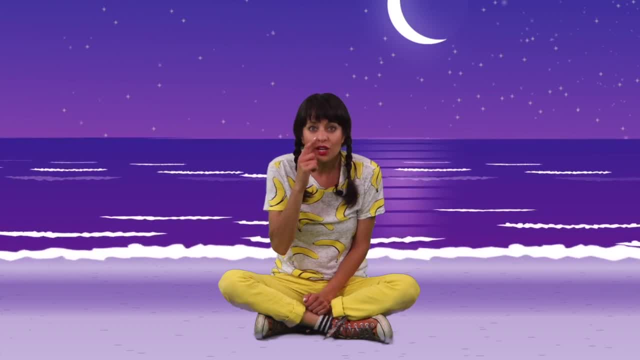 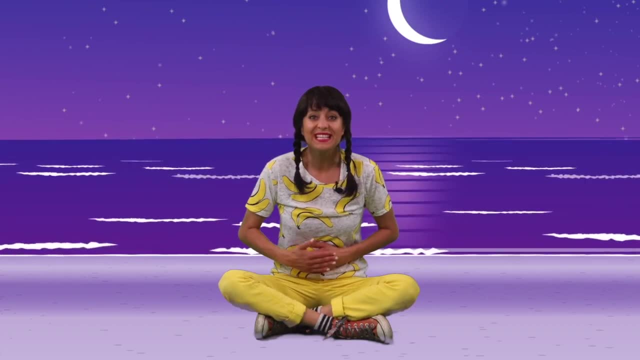 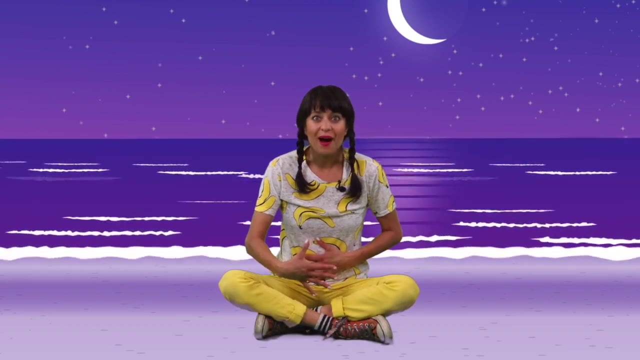 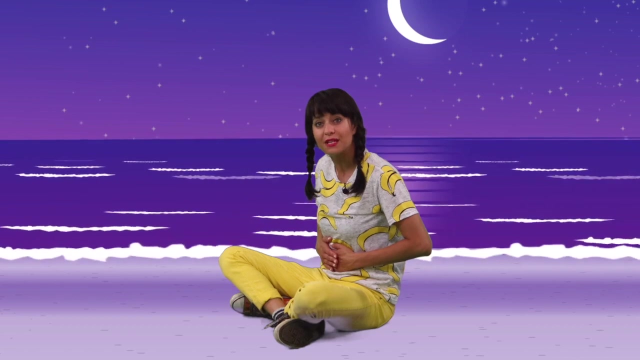 And then breathe it all out just through your nose. That's right. You can even feel the air going down in towards your belly. Try it with me Breathing in. I felt my belly go out And breathe out. Let's try it again. See if you can breathe in, so your belly goes out And breathe it out. 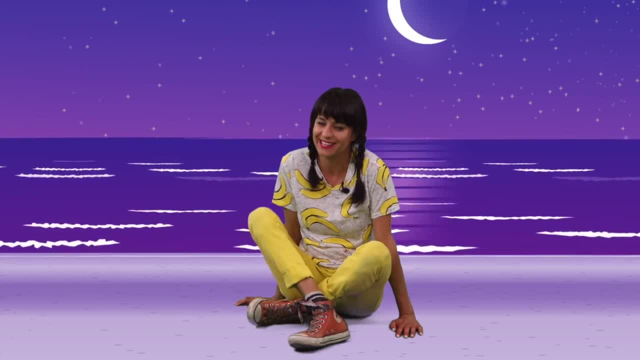 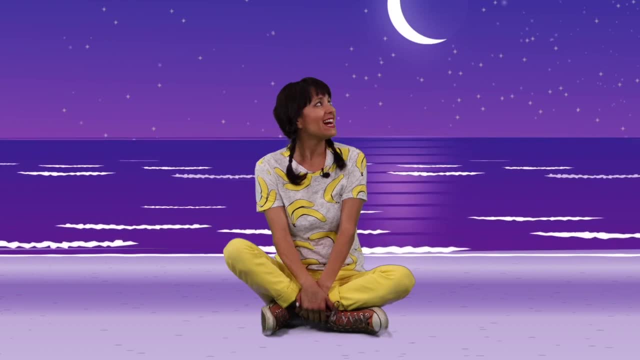 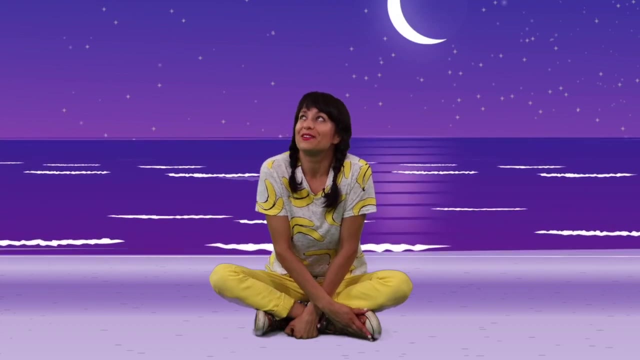 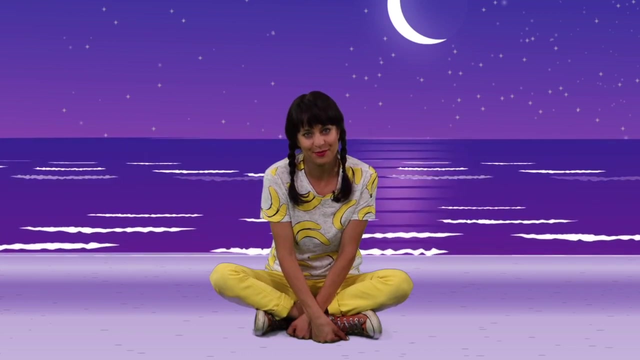 Well, the breathing helps me feel really relaxed and calm, which is good. And now I like to finish off with something that I'm grateful for, And I'm grateful that I'm sitting here on this beach with all of you, underneath a purple sky, with a crescent moon. I'm really grateful to be here tonight with you. What are you grateful for? And it could be someone that you're with right now. 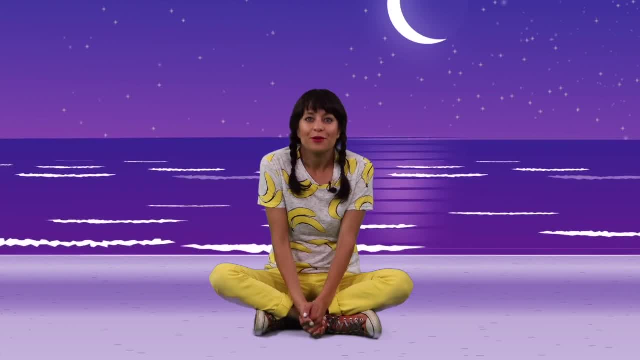 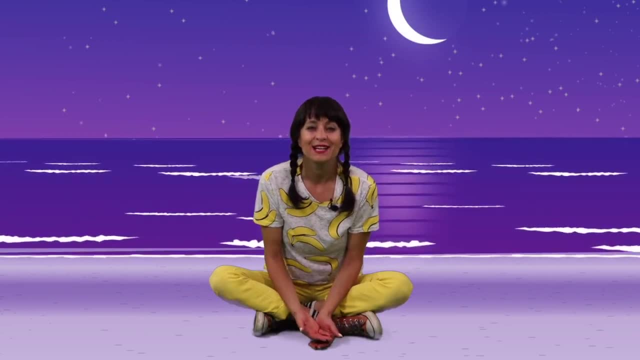 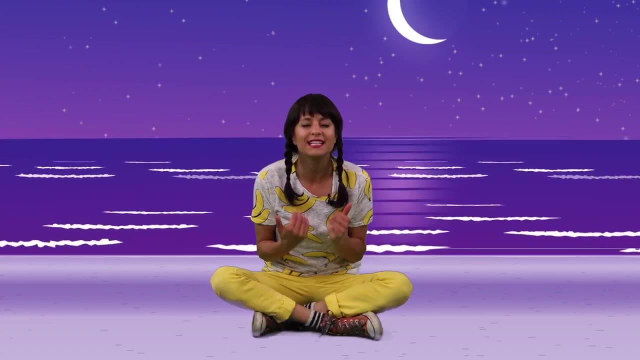 Or your family, Or someone that you love, Maybe your friends. It could be something that you're grateful for, playing outside or playing inside. So close your eyes and think of one thing or two things, however many things that you are grateful for, And go ahead and say it in your mind: I am grateful for. 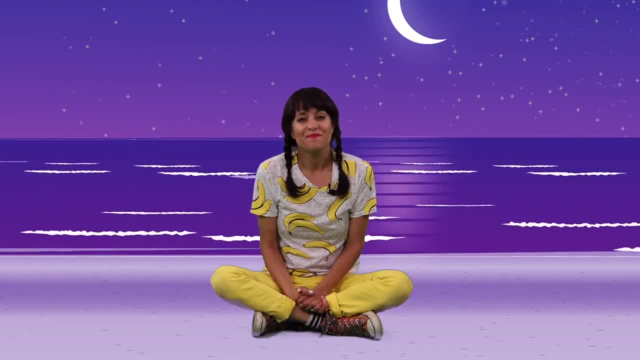 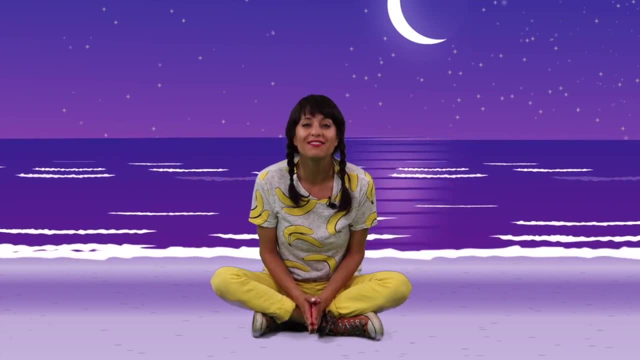 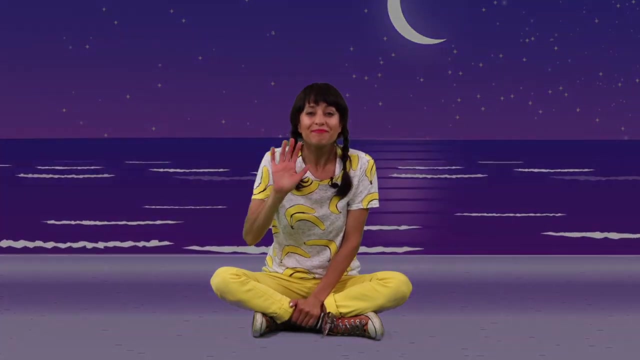 Did you say it Well. thank you for sharing this beautiful night with me And I hope you have a very peaceful and a very relaxing sleep tonight. Bye everybody, Sweet dreams And remember to dream big. Bye Go with yo-yo.